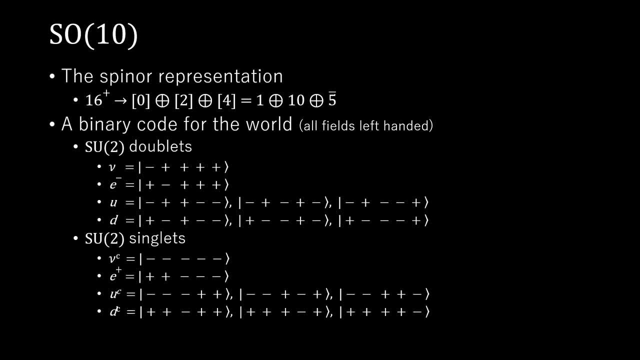 This whale field does not participate in the strong, weak and electromagnetic interactions. Thus we identify the mysterious one as the long-lost left-handed anti-neutrino field By a conjugate transformation. this is equivalent to the right-handed neutrino field. 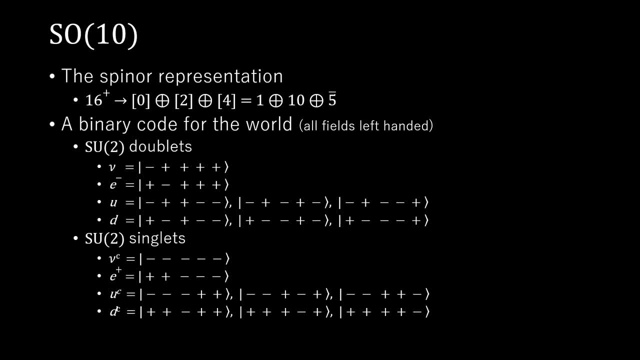 which was missing from the SU-3 cross, SU-2 cross, U-1 theory. In SO-10, the fundamental quarks and leptons are described by a 5-bit binary code. Here's the lineup. We see that the states with 4 pluses and 1 minus describe neutrino electron and anti-D quark. 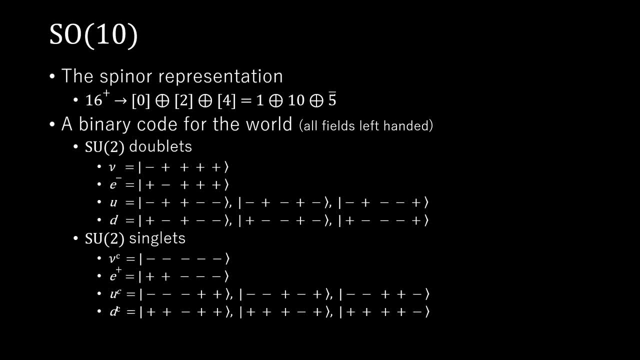 which form the 5 of SU-5.. While the states with 2 pluses and 3 minuses describe U, D, anti-U quarks and positron, which form the 10 of SU-5.. Since the X and hypercharge wire generators. 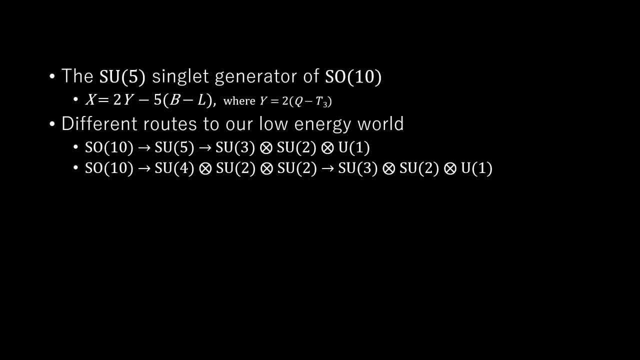 the B minus L, being a linear combination of X and Y, is a generator of SO-10.. This provides another way to see the necessity of the right-handed neutrino field. Remarkably, group theory indicates that the Patti-Salom theory and the Georgi-Glashow theory 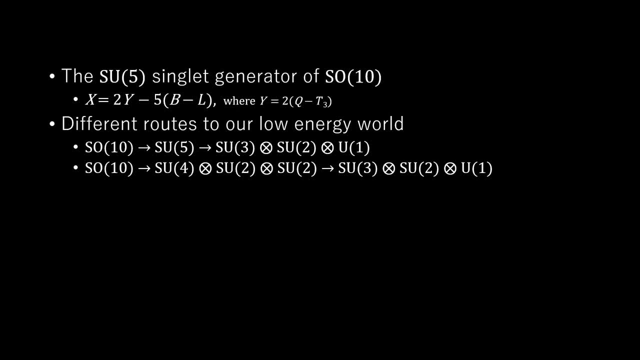 which at the first sight look quite different, may end up being realizations of the same underlying theory. Starting with the grand unified world of SO-10,, there is another route to our life. We are now in the lower-low energy world, other than the first chain of subgroups. 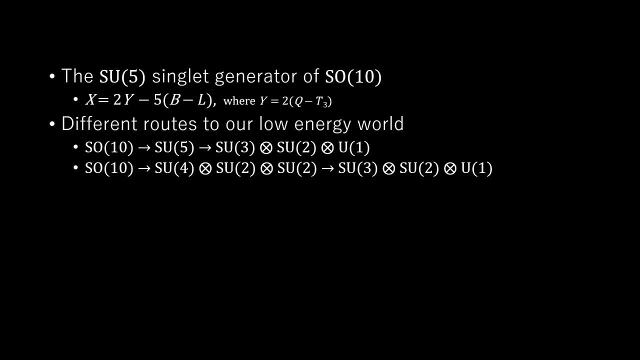 We have discussed SU-5 as a natural subgroup of SO-10, but SO-10 is large enough to have other interesting subgroups. It clearly contains SO-6, cross SO-4.. We know that SO-6 is locally isomorphic to SU-4, which contains SU-3. 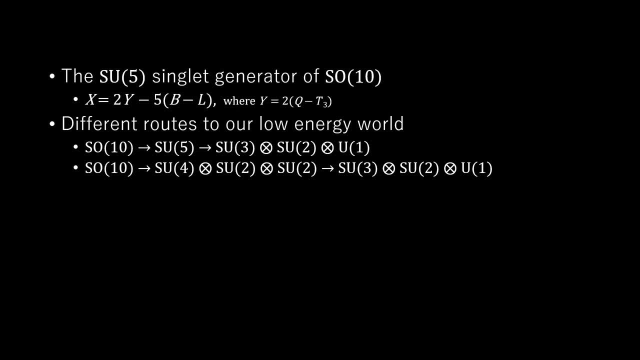 We also know that SO-4 is locally isomorphic to SU-2 cross SU-2, which contains SU-3.. SU2 cross U1.. Thus we can travel an alternate route to the low-energy world going through the second chain of subgroups.